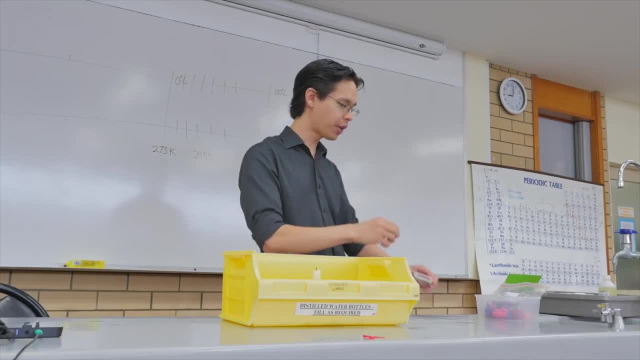 Can you blow out the balloon up a little bit? Because it takes the heat energy, All right. so a balloon that's not as inflated? All right, let's test that idea. It's because it takes the heat energy from the candle and then all of the atoms in the balloon are touched and it's blown out. 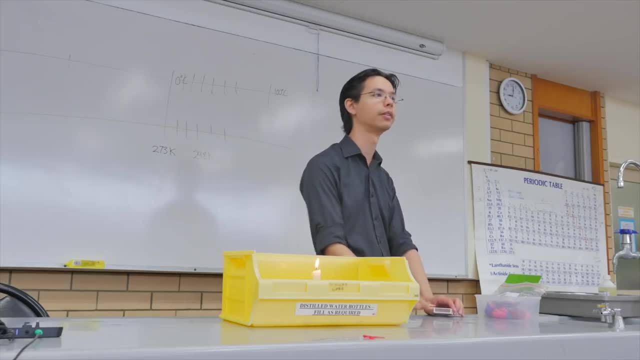 You're the first student to actually give me the reason why it bursts. so well done, Thank you. It is getting the heat energy and the particles on the balloon itself rubber, gain the kinetic energy and they vibrate. They vibrate so much that it weakens the bonds between each other. 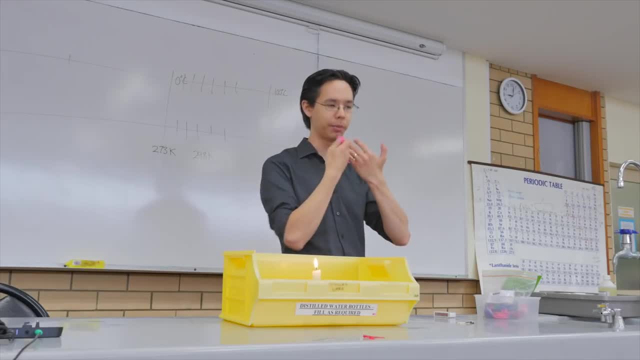 You create a weakness in the rubber and because there's pressure inside, the pressure finds that weakness and bursts through. One more, One more. All right, Yes, So what we're supposed to have on the smaller balloon? It's going to take longer to pop. 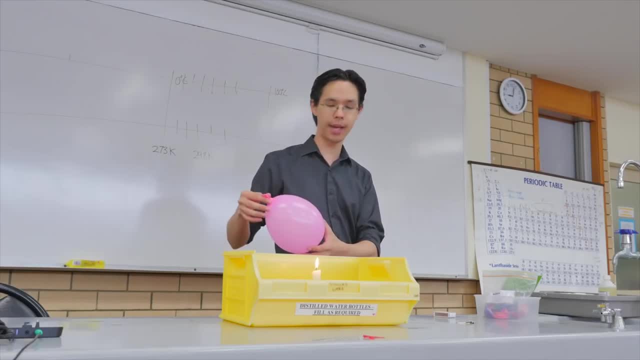 It's going to take longer to pop. Take longer to pop, Yeah, And expand, And expand. All right, Okay, We'll see if we can see an expansion. No, Oh, What's that? What's that? What's that? 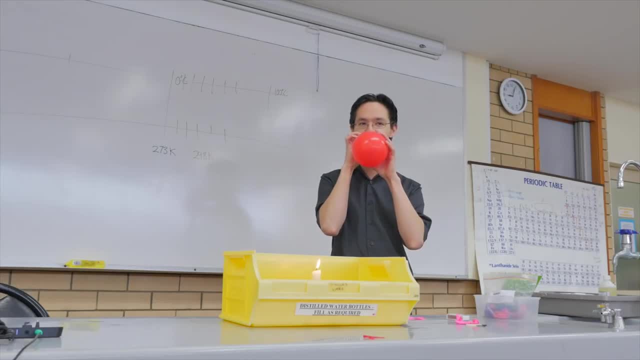 It's quicker, It's quicker, It's just a fun. So yeah, small balloon, Big balloon, Big, big balloon. I reckon bigger is more fun when it bursts. Yeah, yeah, yeah, Tsk, Tsk, Bigger. 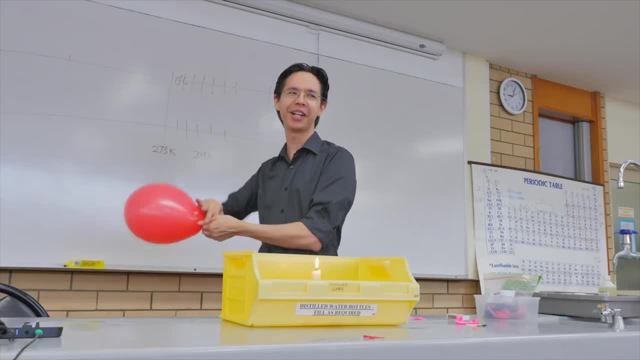 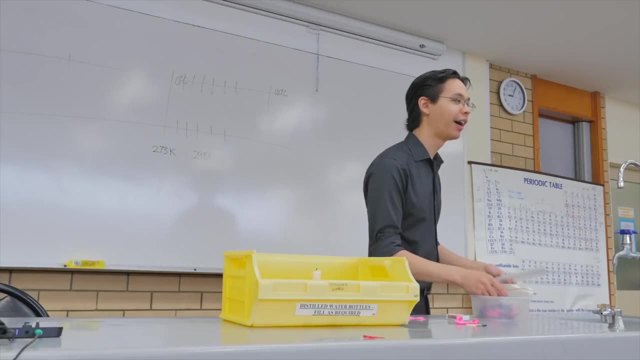 Bigger, Small, Bigger, Bigger, Bigger. That's as far as I'll as I dare to go. That's good. This time I'm going to make a water balloon. As a precaution, I've cleared my bench. 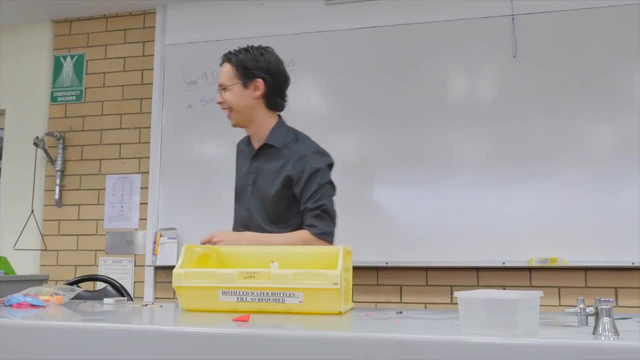 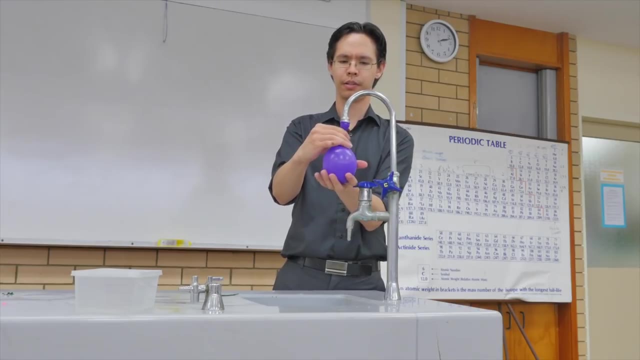 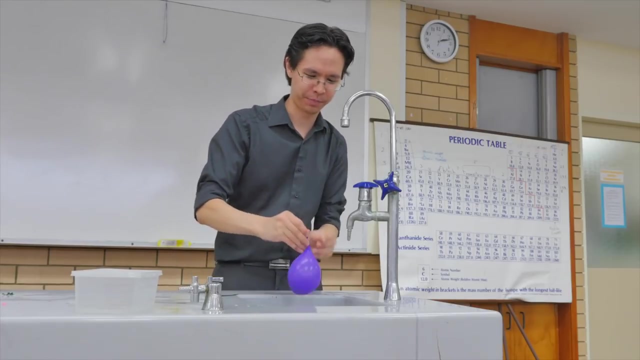 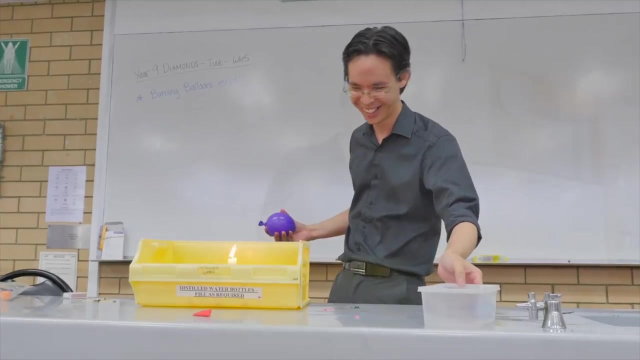 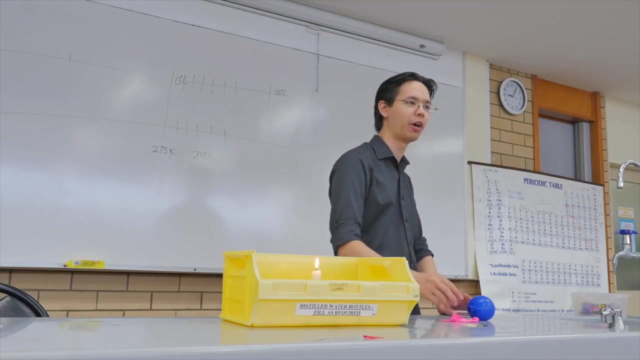 of anything electronic, of anything electronic. i think that'll be enough. now, part of science is to make sure that you have backup plans for any contingencies with manuka or any anything that could go wrong- probably will go wrong, and so i've put this bucket here. i've cleared all my electronics off the bench top. i'm standing over here, you're. 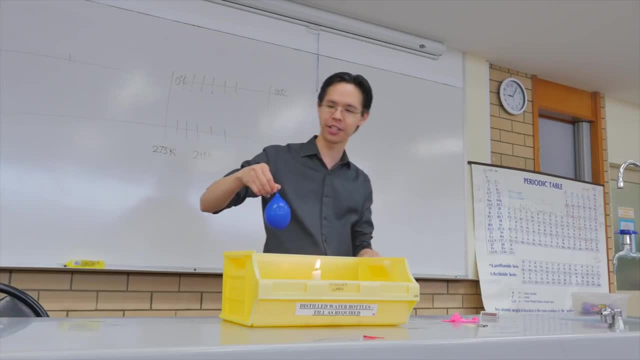 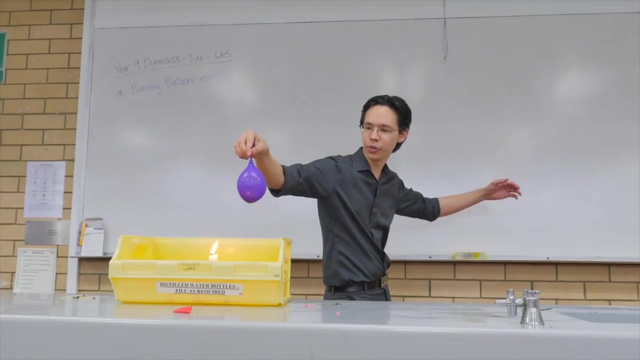 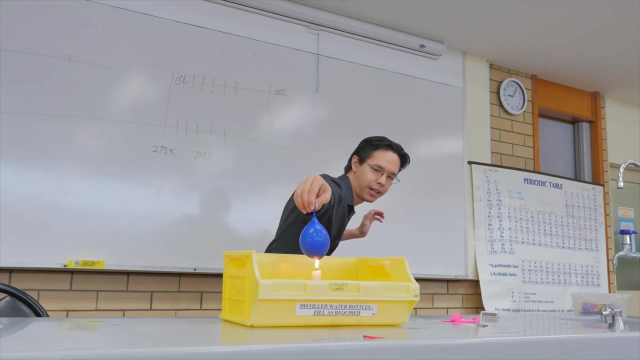 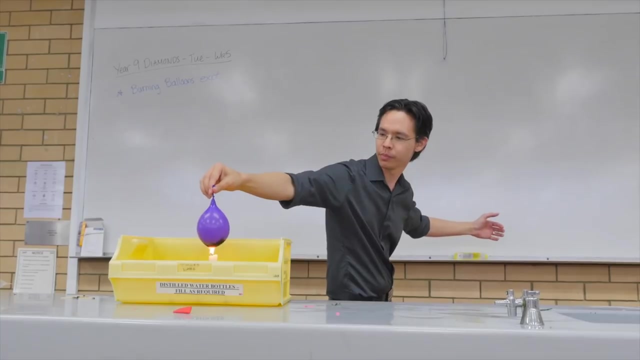 standing over there. my camera is a decent distance away. all right, here we go, ready predictions. all right, here we go. three, two, one, two, one, four, scared though i'm still scared- burning, it's burning. yes, i'm yelling at the camera. so people here that that's closer than the balloon takeover before i. i'm starting to think this is not going to work. 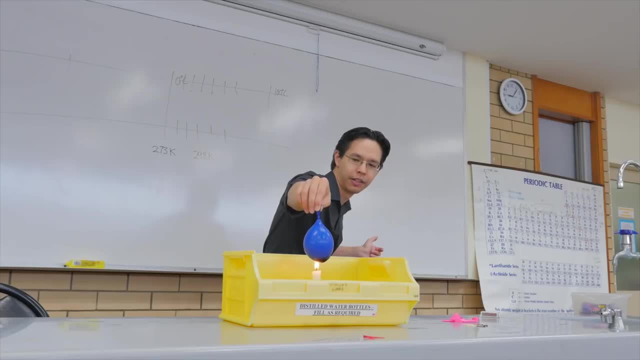 Can I have a volunteer who is brave and who has talented hands? I have talented hands. Alright, I will pick you. Can you please come this way in front of the camera and I want you to be brave and put out your hand and you tell me if it's hot. 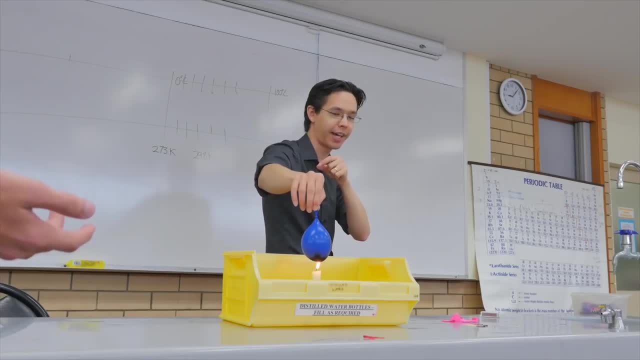 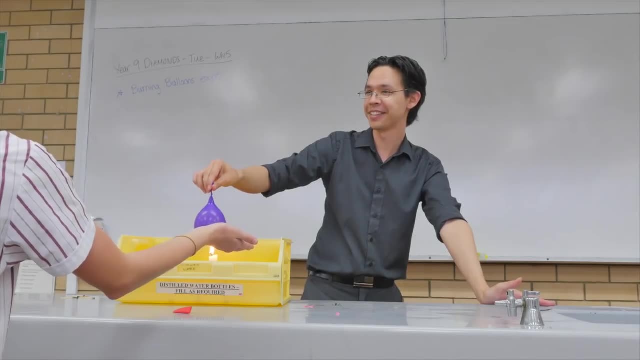 When we hear him scream, we'll know it's hot. Alright, you ready. 3,, 2,, 1.. You don't want to do this, Emi, don't move your head. Alright, if you're scared, I can get the other student to do it. 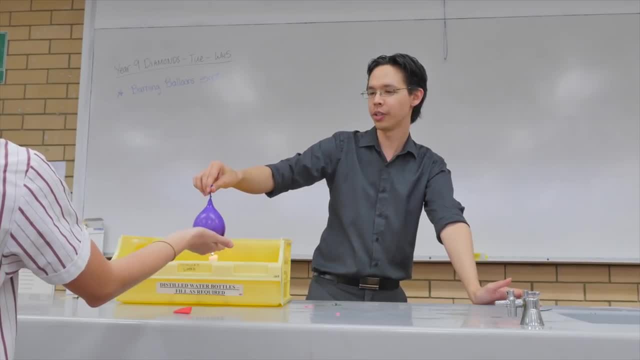 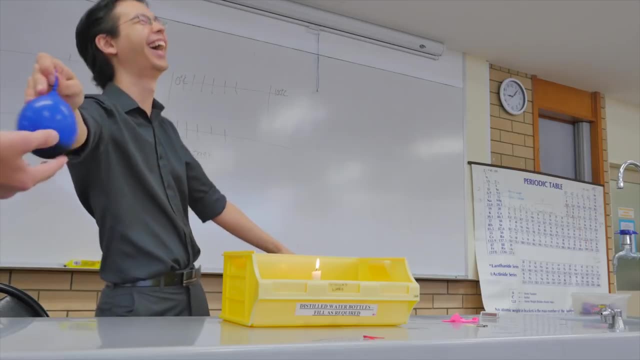 I'll do it. I'll do it. I'll do it. 3,, 2, 1.. Okay, It's slightly warm, but not hot. It's like lukewarm. Yeah, it is about lukewarm. 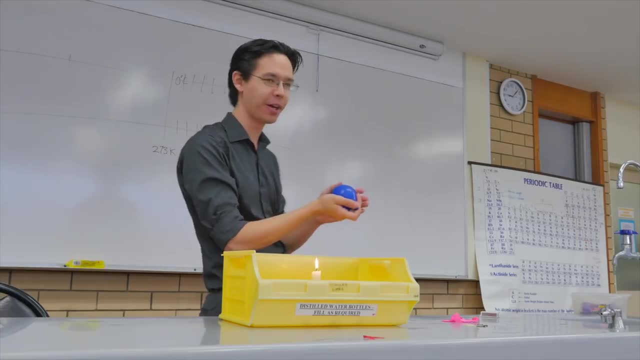 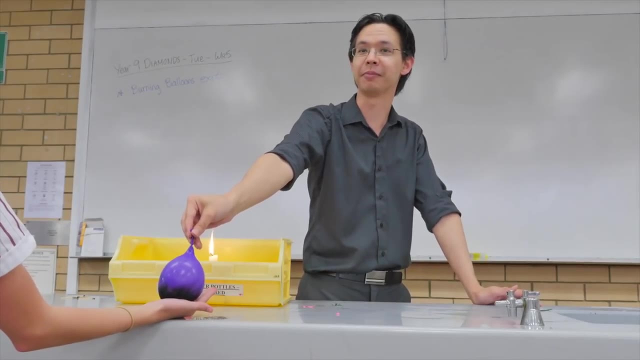 I get the joke, The people on YouTube. his name is Luke. Oh gross. You're so brave, you are great, It's warm. she didn't scream: Let's go again. That is so weird. Alright, now show the camera. 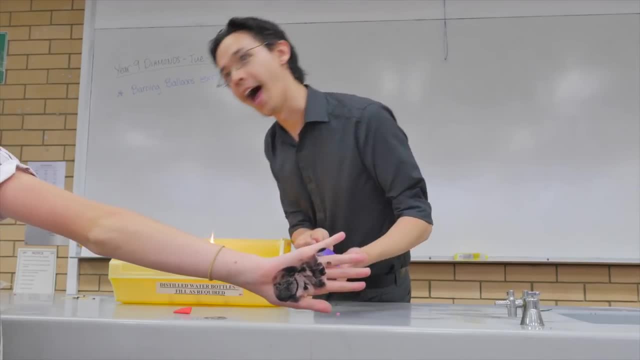 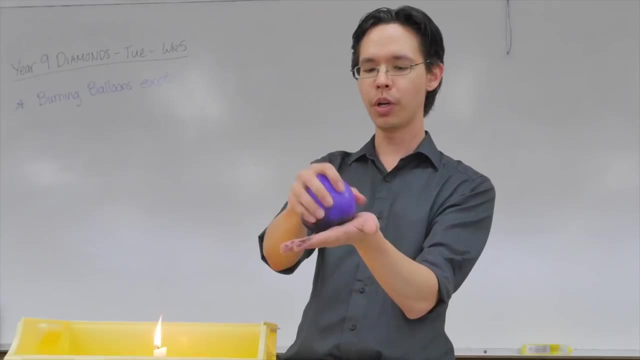 Just put your face where her face is. I didn't do this, so it's like another one of you, Like a tall face appearing on her head. What's on her hand is actually this black stuff. Is it rubber? This is actually soot. 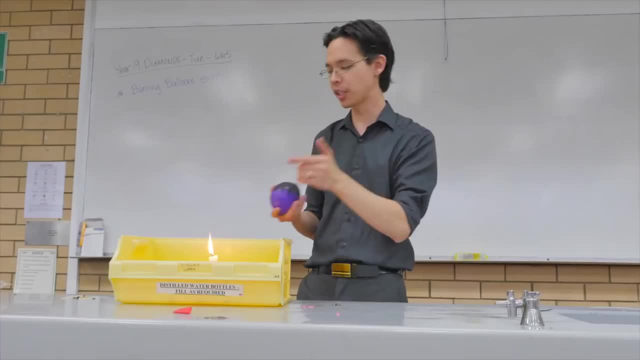 This is carbon. okay, Where's it coming from? It's actually coming from the candle. This candle's made out of paraffin, paraffin wax And wax is made out of carbon atoms, all put linked together. When we apply the flame to it, it vaporizes, turns to a gas. 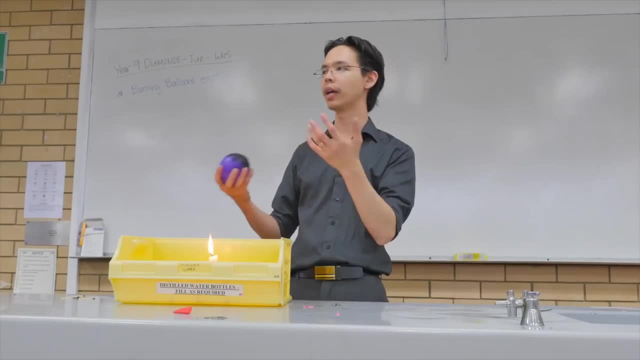 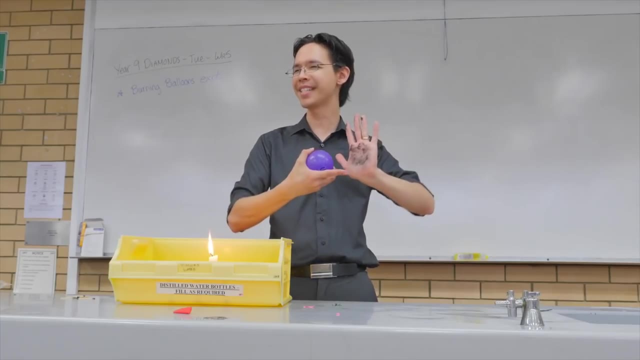 and then the flame is able to combust that into light and carbon dioxide and a little bit of leftovers, That is, the leftovers of a fire. okay, When a fire doesn't have enough oxygen, you get smoke. Can you see the smoke trail? 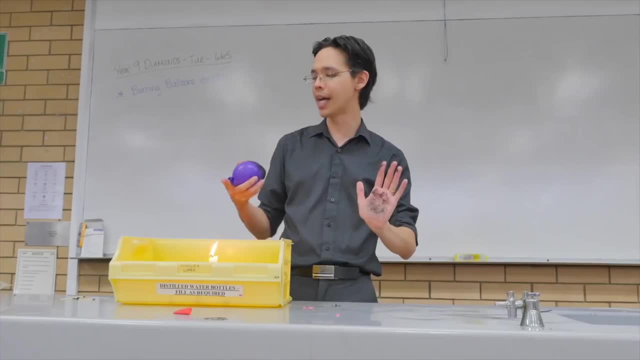 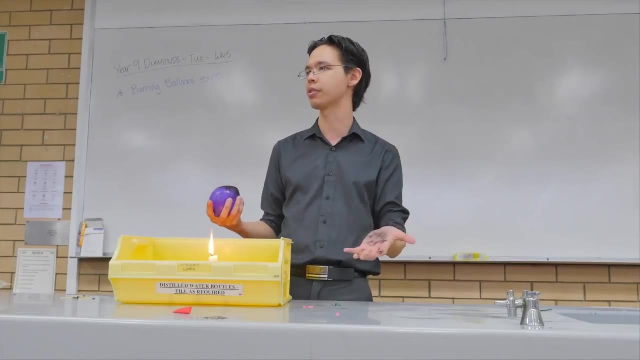 That is leftover carbon that didn't quite burn yet It hasn't quite combusted to carbon dioxide yet. Carbon dioxide, you can't see it right. You breathe it out every single day. it's colorless, But if you've got something that doesn't have oxygen to it, 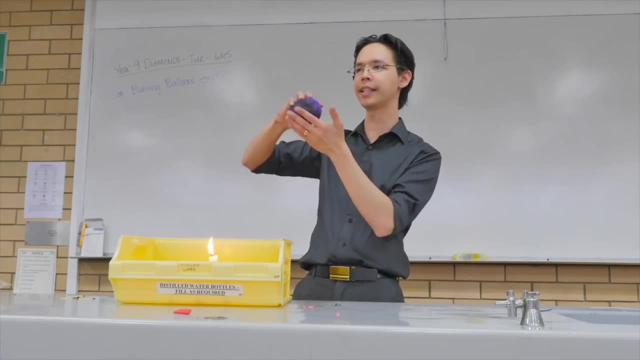 it creates a smoke trail like this. So we've actually collected a whole lot of that soot on the bottom of a balloon. Has it actually burned any of the balloon? Has it burned any of the balloon away? No, It doesn't appear so. 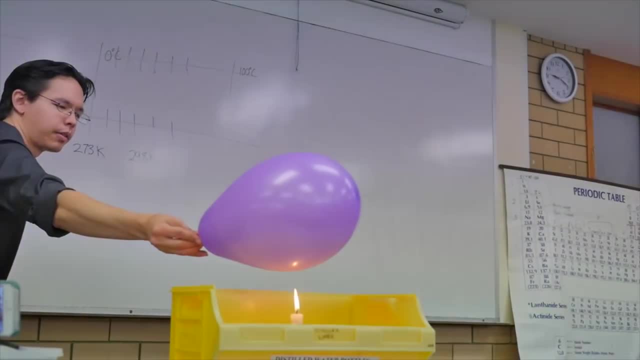 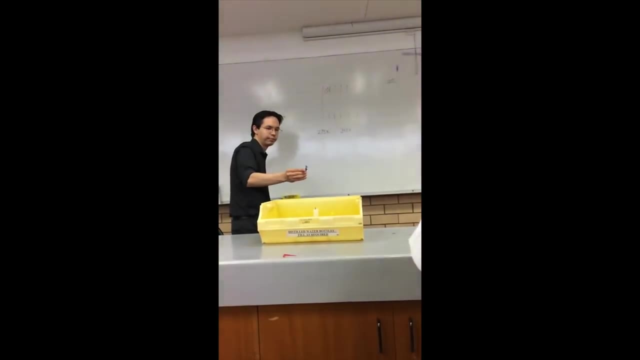 Why do you? How does the water inside absorb the heat? Tell me, Because it's denser than the balloon rubber. It's denser than the balloon rubber. Yeah, It could be right. It could be right. Probably not. 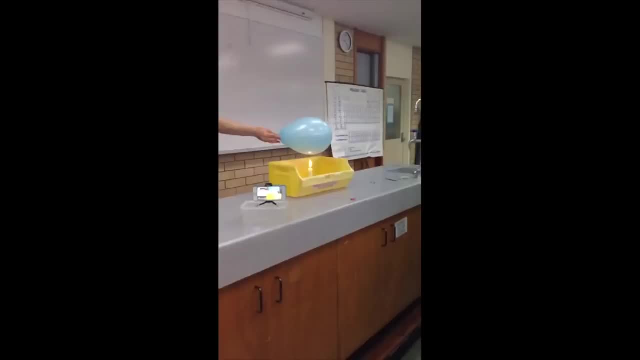 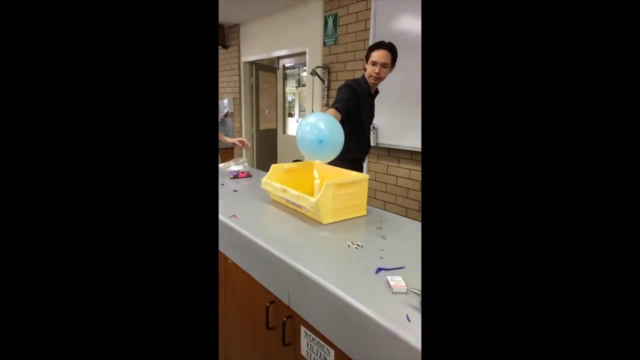 I'm not sure Heat spreads out. How does it spread out? It passes on through all the water. The rubber was the closest bit to the fire, but how does the water actually get that heat? It's because the atoms connect and then it absorbs. 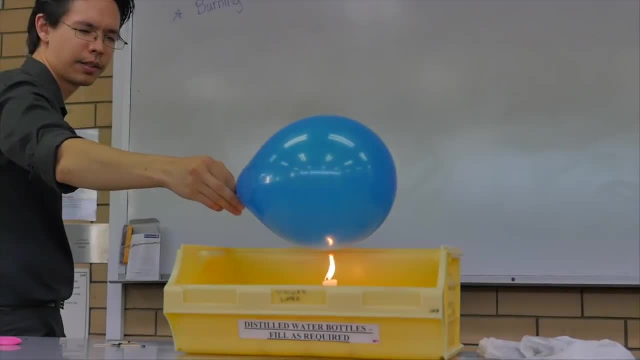 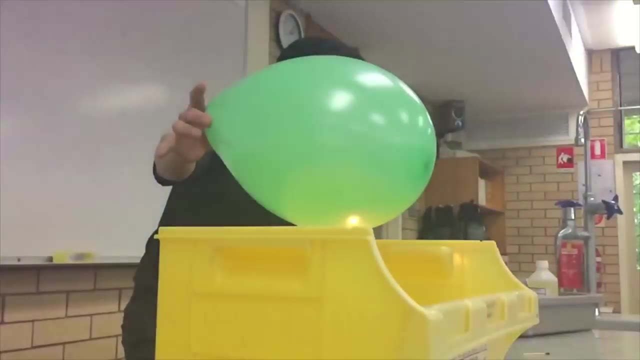 Tell me what you mean by connect. They join together so that when the rubber gets hit, it takes it, the water takes some of the blow, so that, Okay. so I think you're going with that analogy we had before. We're all linking together our arms. 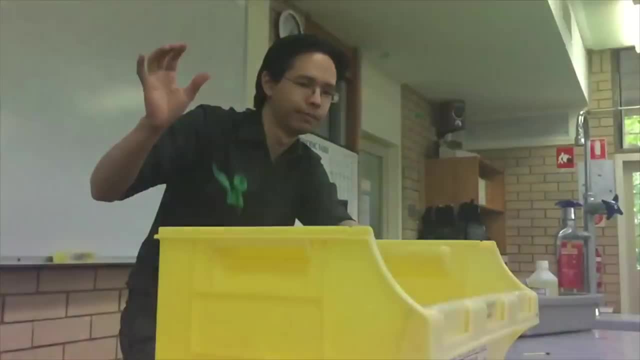 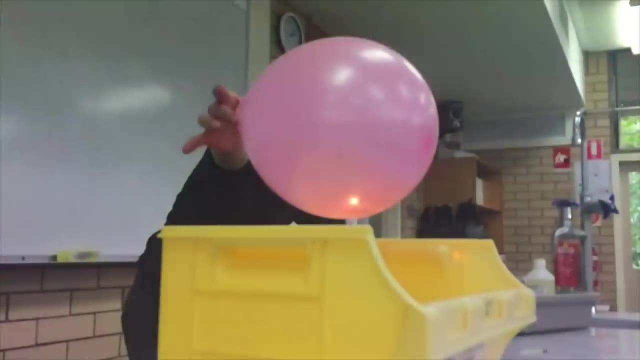 Now we will have linkages between all the atoms that are in the rubber. They are all linking arms, but they're not linking arms to the water molecules inside. but the water molecules are Linked together, Compact, Pressing against each other. 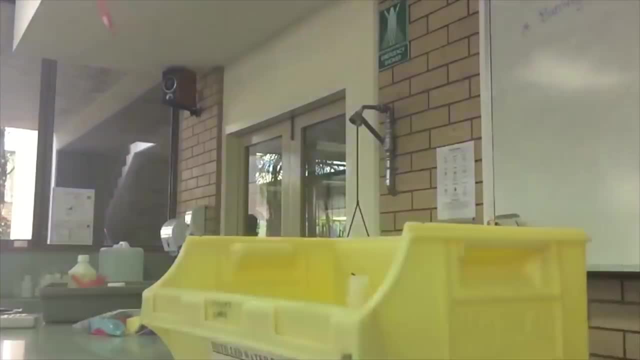 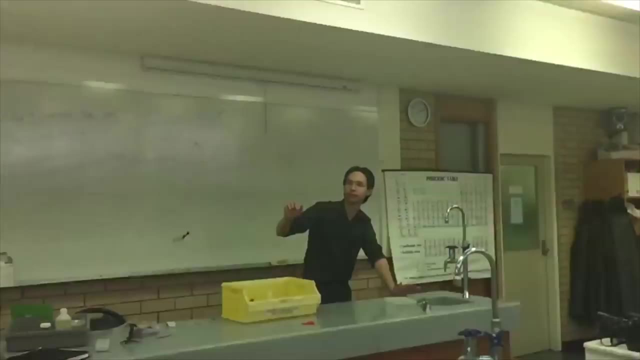 Touching, They're touching, Touching. Aren't the water molecules touching the rubber right now? Yeah, If they're touching, that means they're close enough. Yep, So if I rattle the molecules of the rubber with a bit of fire? 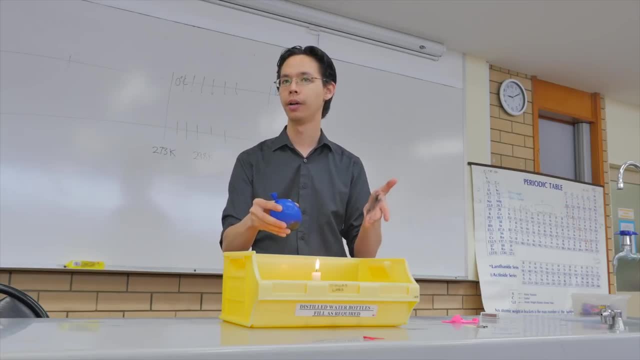 okay, that would then rattle the Water. Okay, Now, why isn't the water boiling? Because the candle is not hot enough. Sorry, Because it doesn't feel like it. There's no air. No, It's not hot enough. 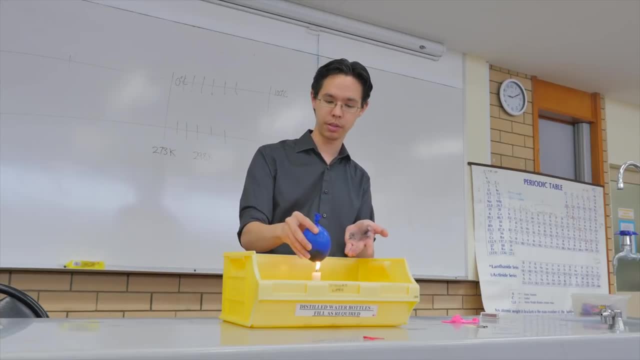 Not hot enough. It could be hot enough. I could boil some water with that if I wanted to, But you have to hold it a lot longer, A lot longer. Why does it have to be there for quite a long time? Because it's a really small flame. 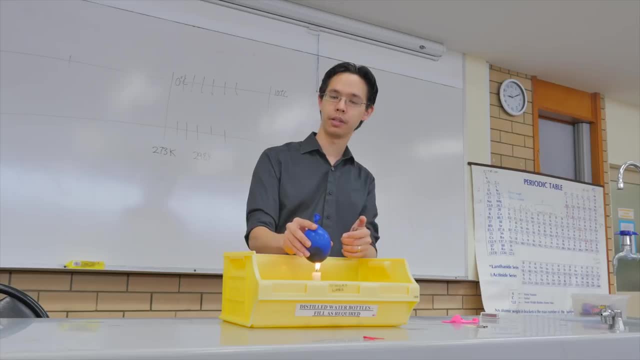 Oh, oh, Because the flame is just like hitting, like it needs to be all around the balloon, All around the balloon. Yeah, It needs to give time for the water, because the heat will only be in some parts. It's only affecting a little portion of the balloon. 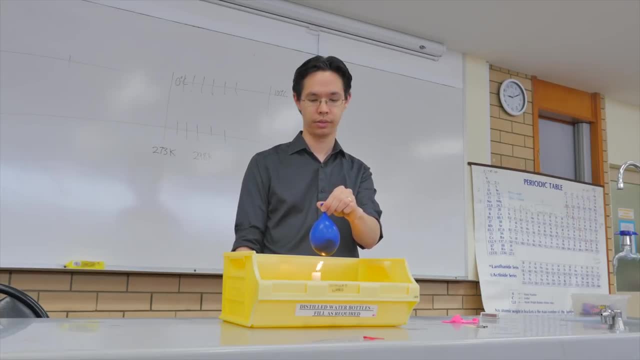 Okay, Oh wait, Is it? because it's only at the base of the balloon? and? But doesn't, don't you boil water with a pot on the stove? Yeah, And then stop heating from the bottom? Yeah, but you have to let. 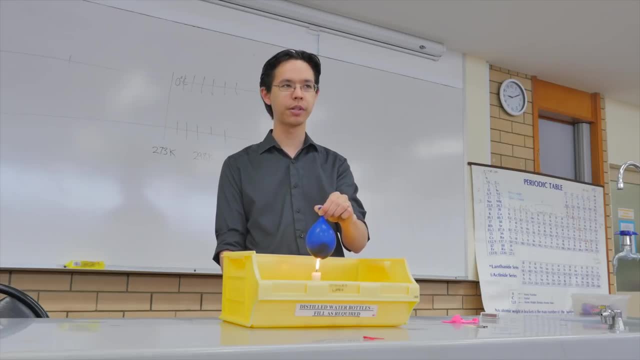 It circulates. Give it time so that it can reach some degree. Just putting it in like a circle so that gets a lot more heat. A bigger, a bigger base of fire would definitely distribute the heat more evenly, but it wouldn't encourage it to boil any faster than a single flame. 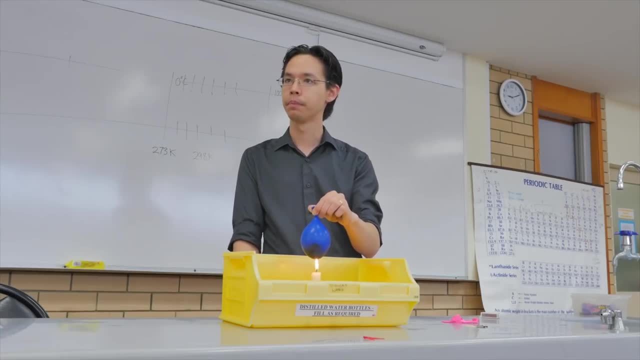 Um, rubber isn't a big conductor of heat and doesn't spread out as much as like steel. Yeah, I love the Ah he's mentioning. he's mentioning thermal conductors. Okay, Rubber is usually not a very good conductor of heat. 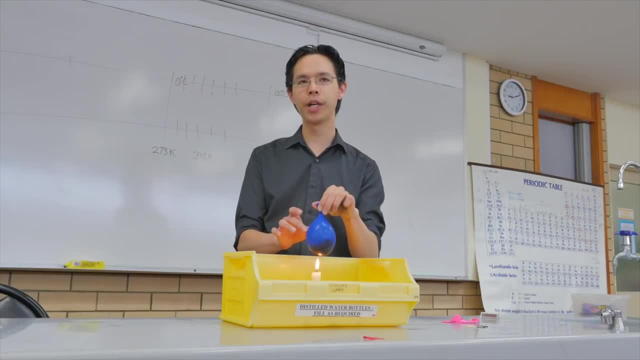 Not. not as well as as steel does. The reason why it's not boiling is that for the given amount of heat, I have to heat up a whole lot of water molecules. Yeah, Okay. So every time I apply heat from the bottom, 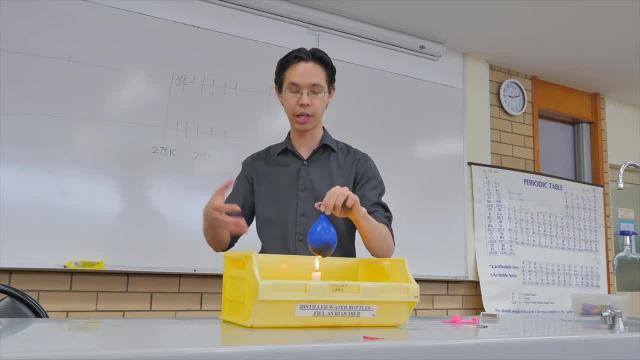 the rubber gets extremely hot, vibrates a lot, vibrates the nearby water molecules on the bottom and those water molecules, those water molecules, share it amongst each other, all of them inside the water balloon And that's a lot of water. 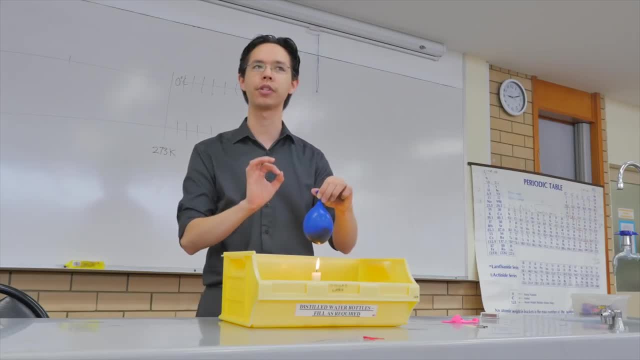 It's kind of like now this is a bad analogy, but just think, go with me for a second. You know how like kids kind of get hyper on sugar. Oh, that's me, Okay. Oh that's you, All right.